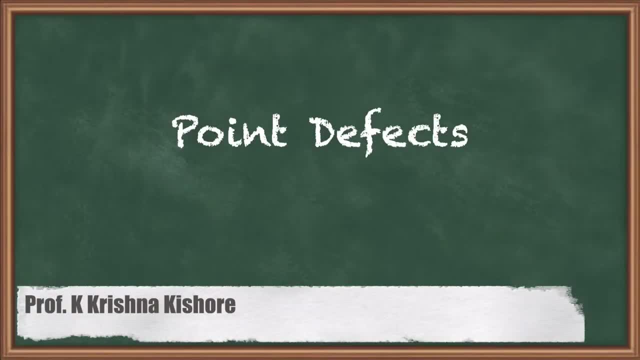 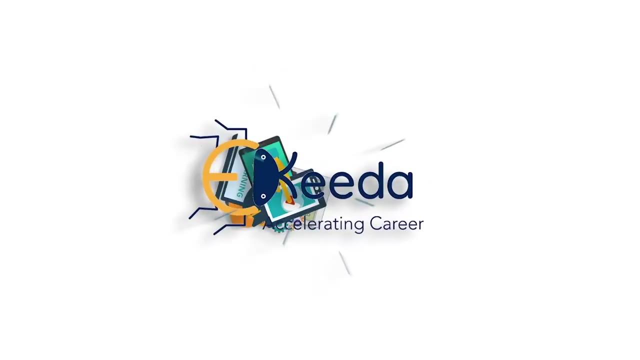 Hi students, I am Kakarla Krishnakishore, Mechanical Engineer. In this session we are going to discuss the first defect in lattice imperfection, that is, point defect. Now let us discuss the point defect. Before going to discuss the point defect, just observe the detailed classification of the. 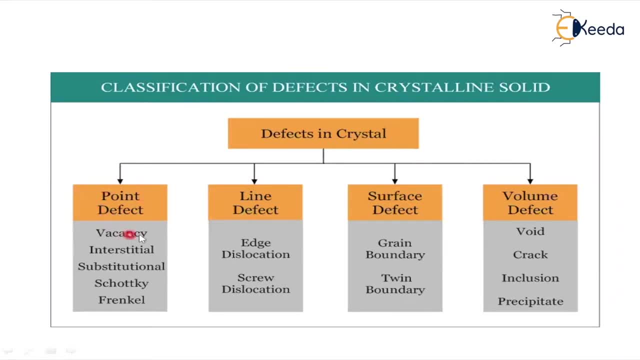 crystal. so now you are observing point, defect line, defect surface and volume. these are the various states. therefore, in the previous research I have shown that the 500 mT I wanted to may be observed in various crystalline soils. Now in this session we are going to discuss 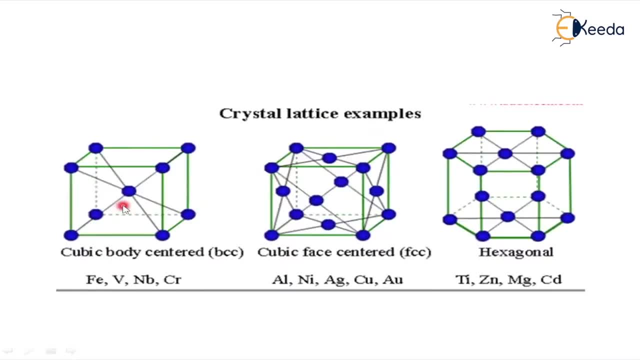 the point of it Here. observe the various crystals here. This is body centered cubic structure. This is face centered cubic structure. This is hexagonal structure. In all these structures you are observing various atoms placed at different positions, Maybe at corner, maybe center, maybe on the face. If any one atom is missed here, automatically the property. 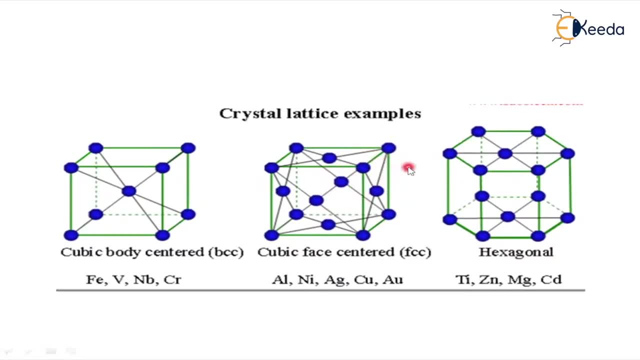 may have some effect. So this is very, very important. So that means point debates are very, very important to understand and to identify or to analyze the properties and the analysis of the crystalline solids. So that means if any atom is missed from the place, we have to identify, we have to analyze why the particular atom is missed. 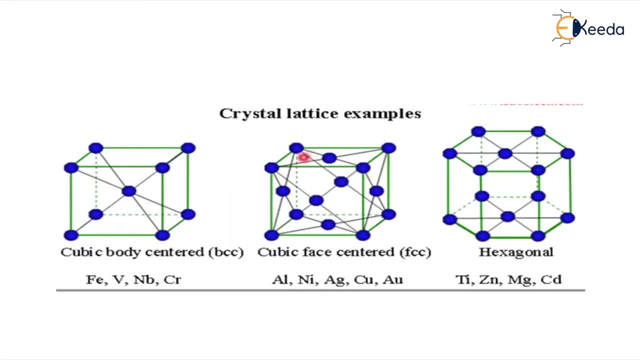 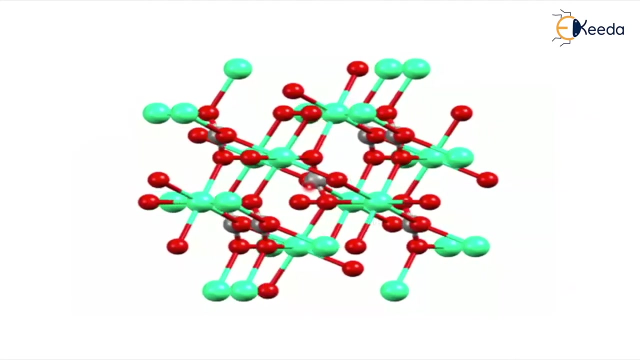 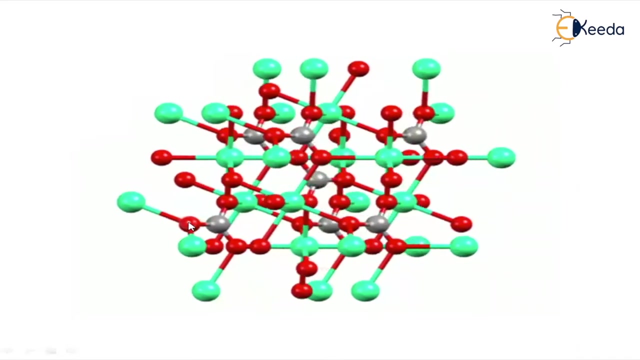 from the place Why the atoms are, occupies another place. So all these analysis may be done after understanding the point debates. So that's why this point debate analysis is very, very important. Now we are going to discuss this point debate individually. Now see the pattern here. This pattern, if you observe, various atoms are combined like 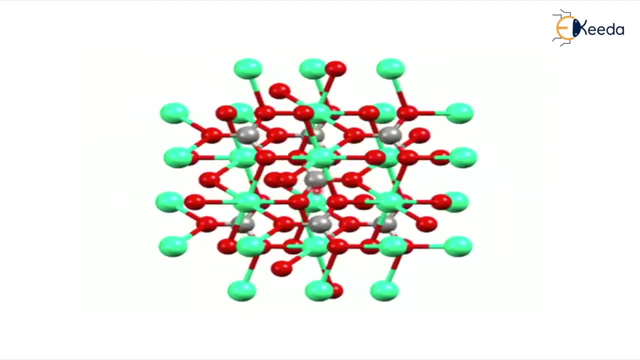 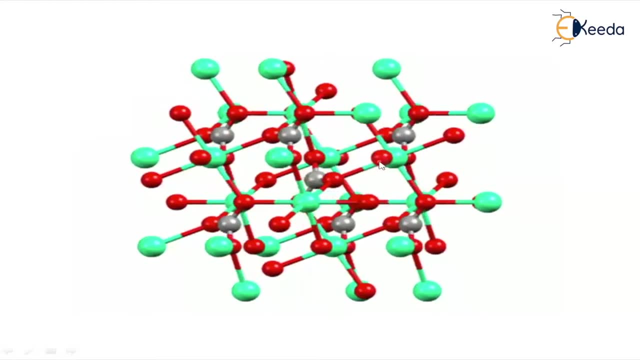 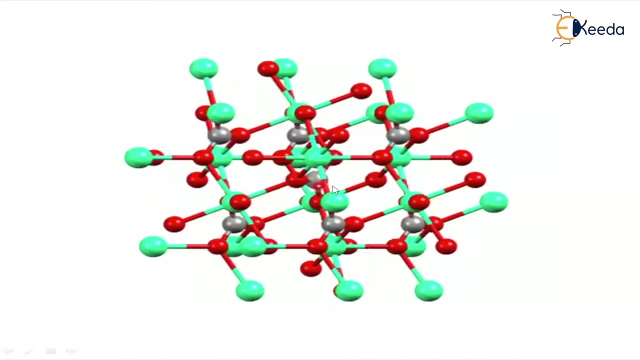 this: If any one atom is missed here, the total crystal structure may have disturbance in exhibiting their properties. So that's why each and every atom is important. If you observe carefully, all atoms are connected and interlinked with each other. So this is. 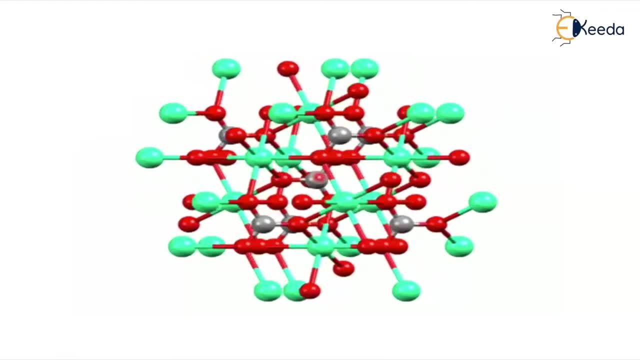 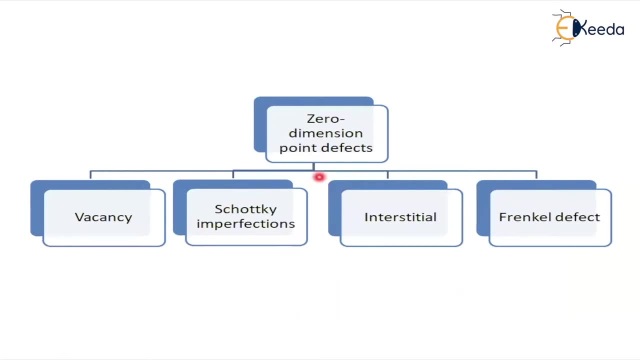 why each and every atom is very, very important in the crystal solid structure. Now the following is the classification of zero dimension or point debate. It is further classified as vacancy, scotky imperfections, interstitial imperfections and Frenkel imperfections. Now 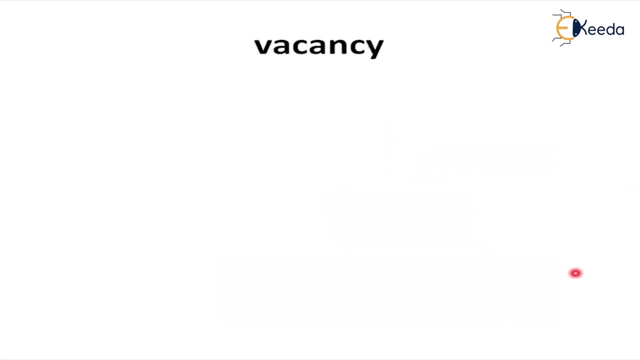 type in point effect. so that is vacancy. so what is vacancy here? first observe the definition. here vacancy is defined as it is produced when an atom is missing from its original site. that means if any one atom is missing from the original site, we can say that it is vacancy defect. so vacancy creates an. 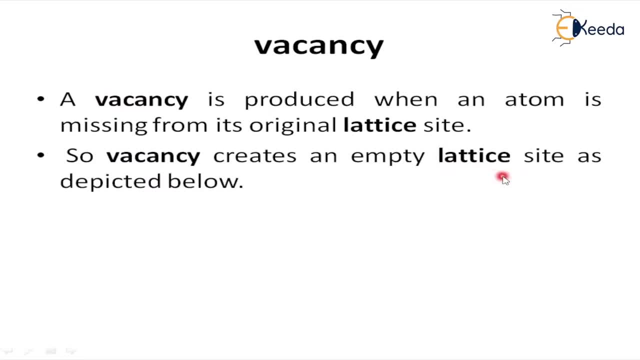 empty lattice. so that means empty space side. that is called as a side lattice side as depicted below. see the picture here. if you observe, this place is an empty place which can be represented as vacancy. now see the next slide here. this sentence is very, very important: missing atom at a certain crystal lattice. 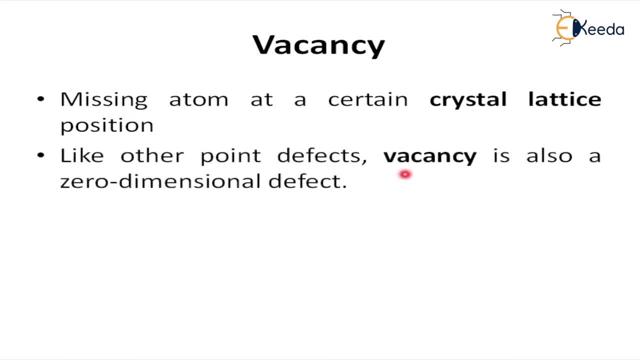 position. like other point defects, vacancy is also a zero dimensional defect. what do you mean by zero dimensional defect? zero dimensional defect means here the point atom or the atom is missing only from one place here, so that's why it is called as a zero dimensional defect. now observe the next sentence here. vacancy defect puts the: 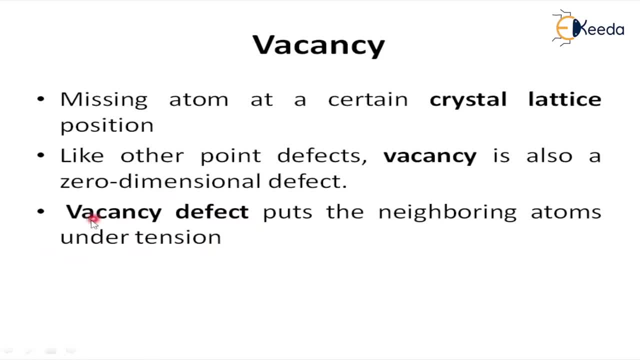 neighboring atoms under tension. what it means here: if any one atom is missing from the place, automatically the other atoms. now I will show the picture in the next slide. please observe the sentence carefully. it gives the tension. why it gives the tension, why the tension may be happened. please observe here now this is: 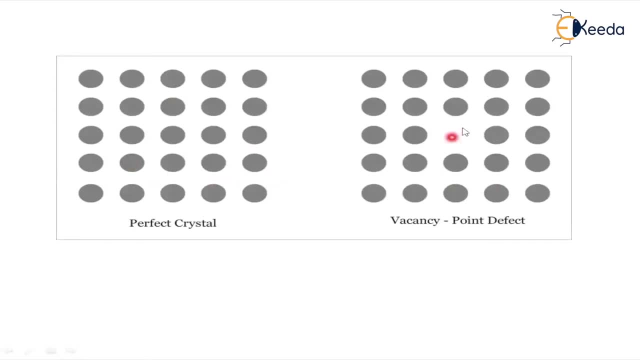 the perfect crystal. this is the vacancy here. one atom is missed and the other atom is missing. if any one atom is missing here, automatically this one atom wants to occupy this position. this atom also wants to occupy all these atoms, all these surrounded atoms. wants to occupy this vacancy position automatically. this place is under tension, so that means vacancy creates. 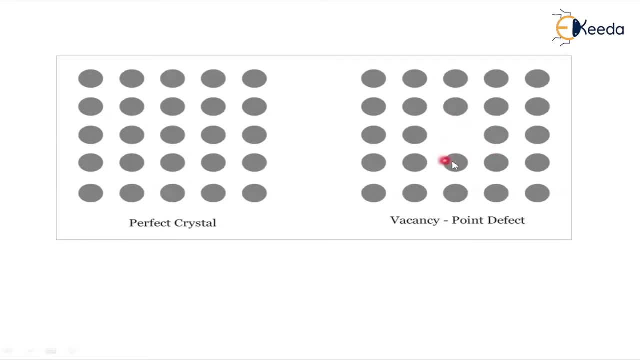 creates a tension in the crystalline solids and that gives the tension. that means the vacancy is under tension about this viscous is under the Anatolian state which is called daytime system. one atom comes under tension and get is a water space inside the liquid space. 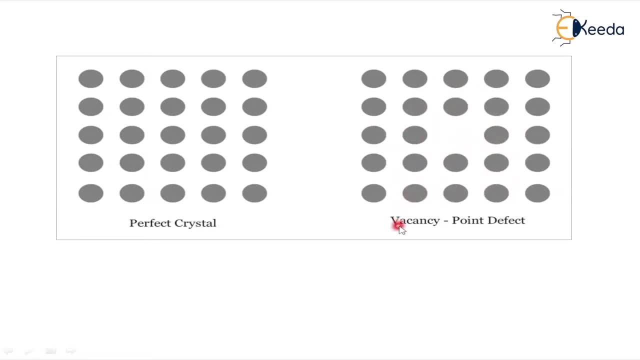 itself is a imperfection. so that's why this vacancy is very, very important. in point effects, we have to identify how many vacancies are there in a particular material. the analysis is very, very important in the crystalline solids. now let us discuss why and where the vacancies can be formed. 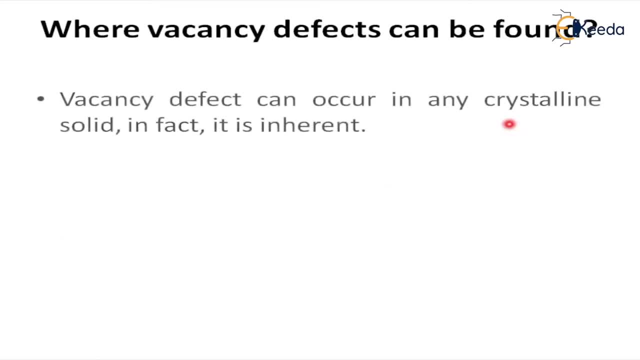 please observe. the first point is vacancy defect can occur in any crystalline solid. this is very, very important. so that means not only in one material. we cannot say that we can see is observed in one particular material, maybe aluminium, maybe copper. know it may be observed in. 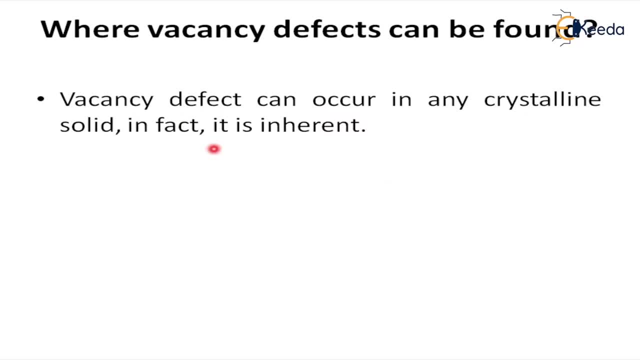 any material. so that is very, very important. the next important point is: any material okay, but Academy temperature is above absolute zero temperature- that is very, very important- can contain vacancies. so that means at zero temperature vacancy may not be happened, may not be observed, may not be generated. but if the temperature 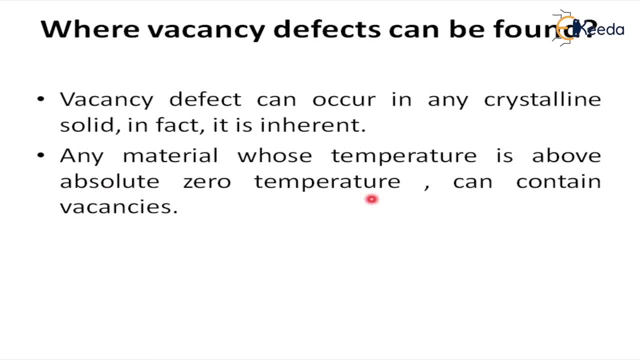 increases automatically. the vacancy may be observed in a crystalline solid. so here we can say in another words: vacancy is directly proportional to the temperature. that is very, very important here. so here the temperature plays a vital role in creating vacancy defect. now the next sentence. if you observe, 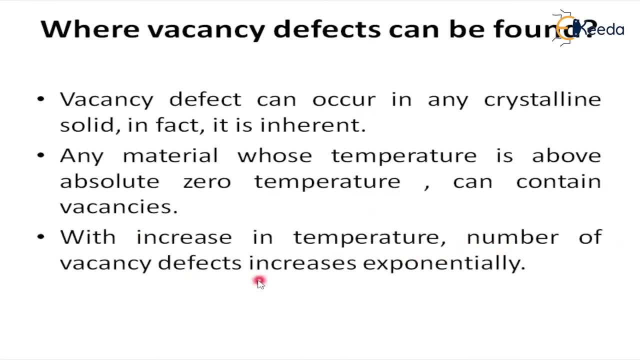 with the increasing temperature number of vacancy defects increases exponentially. here not only the temperature, here the number of vacancy defects. so that means by increasing the temperature if only few vacancies are observed, then it is okay. but here you can say that vacancy defect increases exponentially. this is a problem for any material. the 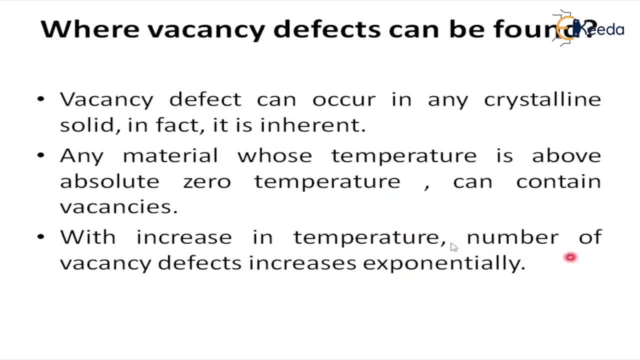 vacancies are increasing exponentially, automatically material loses its strength. if the material loses its strength, we cannot utilize that material for the final purpose. so that's why, before going to utilize any material, identify whether the material is having vacancy defects or not. if the vacancy defects are existed, how many number of vacancies are existed? how many atoms are misplaced or ions are? 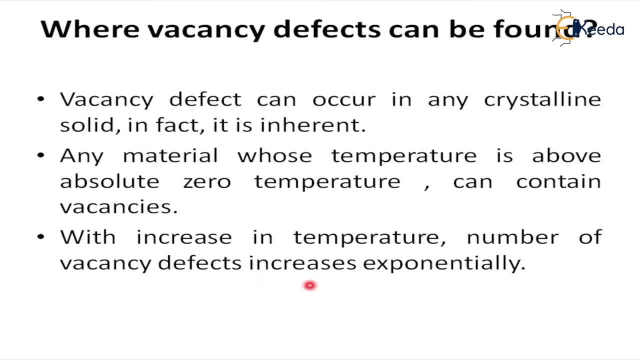 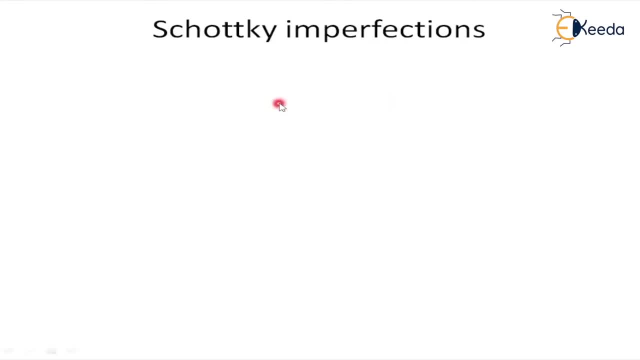 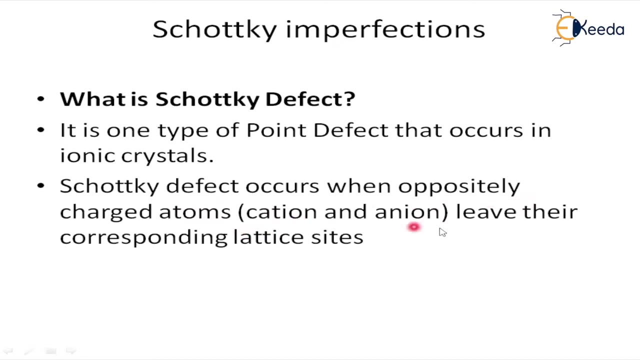 misplaced. so this is very, very important in point defect. the next point defect is scottky imperfection. so what is scottky defect? if you observe, it is the one type of point defect that occurs in any ionic crystal. but the observe, if you observe carefully, cation and anion, if both the 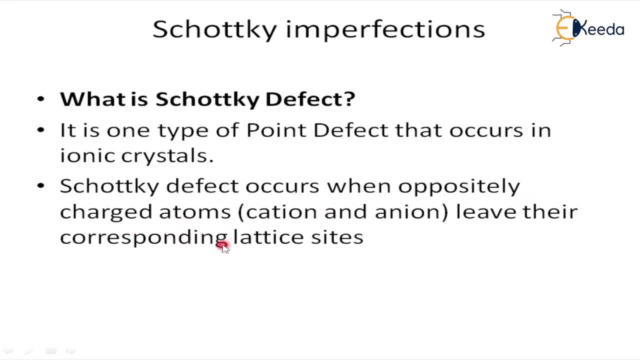 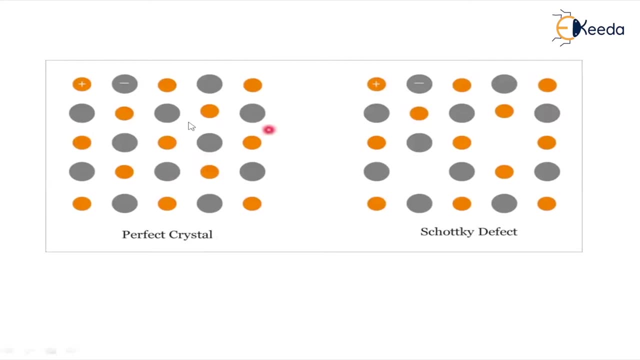 cation and anion miss from the regular side. we can say that it is a scottky defect. please observe the picture here. observe the left picture is a perfect crystal made with cation and anions here. two places are miss here: small ion and bigger ion, if both are miss from. 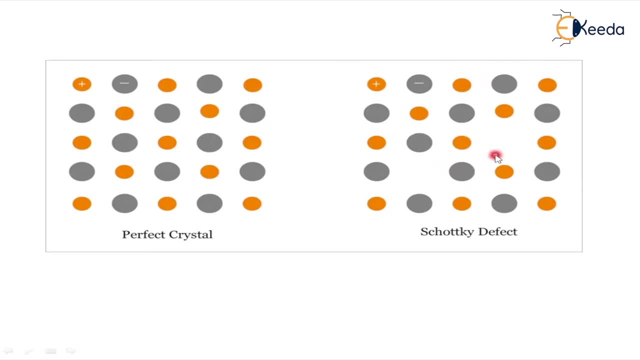 the place automatically. we can say that it is a scottky defect in crystalline solid. so that means if both cation and anion are misplaced, automatically we could say that it is a scottky defect because by because of the movement andины of queste. 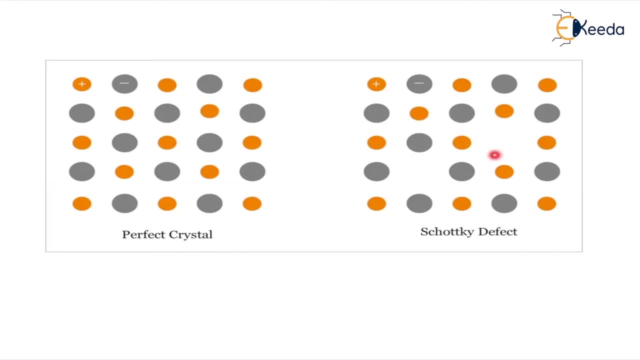 ion and anion is misplaced from the crystalline solid. because of this we can conclude that here the material property may have some changes. so that's why you have to identify. before going to utilize any particular material we must identify what type of defect is observed in. 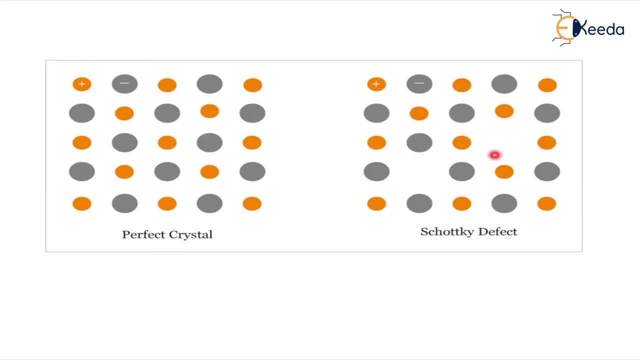 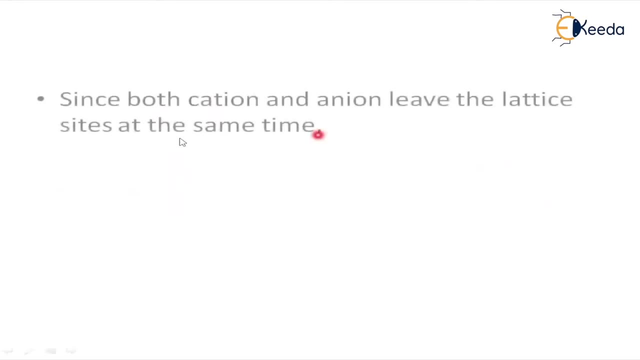 that material, whether it is a scott key defect or vacancy defect. here the main problem. what is the main problem with scott key defect? if you observe, that means both the cation and anion leave the lattice size at the same time. because of this, the main problem is overall electrical. 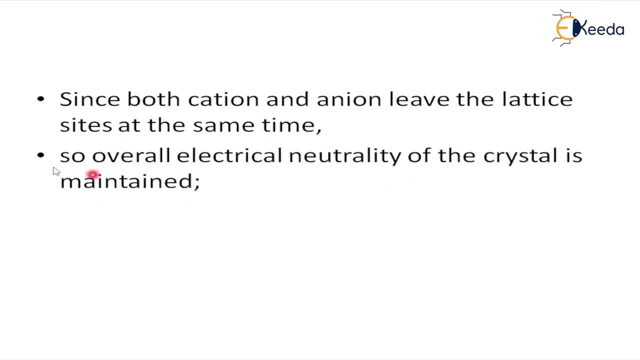 neutrality of the crystal is maintained here. if both the anion and cation are misplaced from the place. from the side we can say that overall electrical neutrality. the balance may be loosed by the crystalline solid. however, the density reduces. this is another problem. because of the scott key defect. density reduces because of all these vacancies. now here examples where: 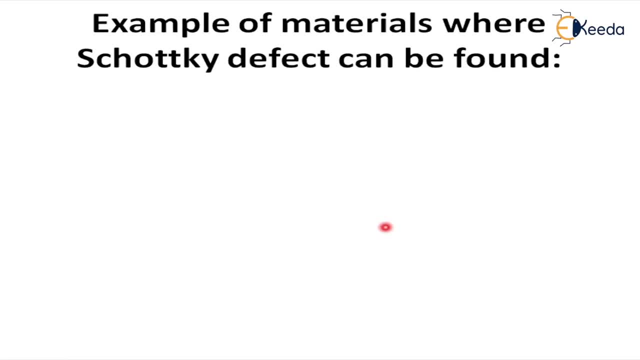 what are the various materials that you are observing, the regular scott key defects? one is sodium chloride and another one is a potassium chloride and potassium bromide and silver bromide, cerium dioxide and thorium dioxide. these are only some examples in which we can observe scott key defect. the next point defect is interstitial defect. what 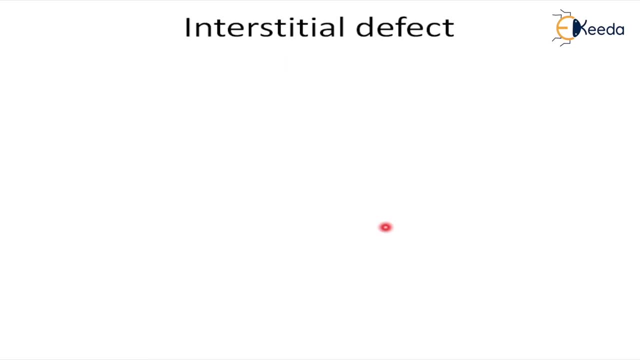 is this defect, when it occurs? this these questions has to be answered here. what do you mean by interstitial? let me discuss the definition first. an interstitial defect occurs when an atom takes the interstitial position of the lattice structure. so that means here the definition concentrating on interstitial position. 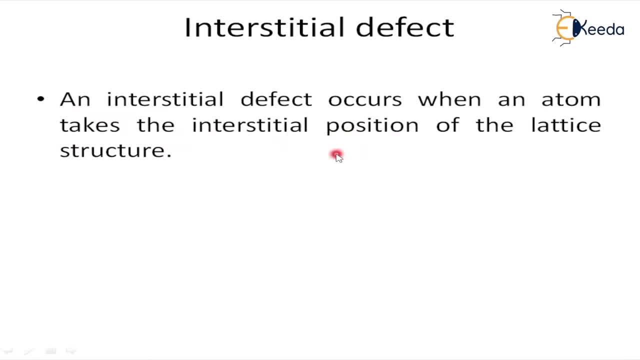 what do you mean by interstitial position? the interstitial position means that the, the place at which are, we can say that it is a void space, wide space. here the interstitial atom may be of the same crystal or of a form material. this is the another information which are related to interstitial defect. so that means 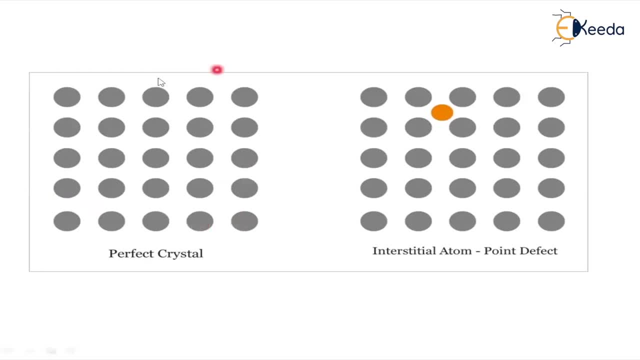 the interstitial atom may be of the same crystal or of a form material. let me discuss with the help of a picture here. yes, please observe the picture here. include theación here carefully. here, this is a perfect crystal. this is another crystal in which the autumn occupies interstitial position. this is the interstitial position. this 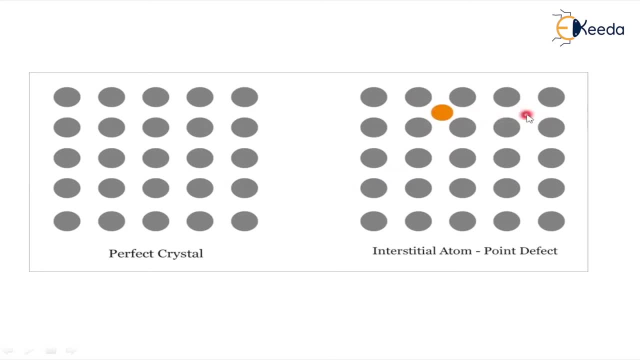 is another interstitial position. this is another interstitial position. if a foreign autumn- maybe for not maybe the same autumn- if occupies interstitial space, then we can say that it is a substitution or interstitial effect. here the same autumn, maybe the hard Solutions and Explanation on Shrav-Brahmi. 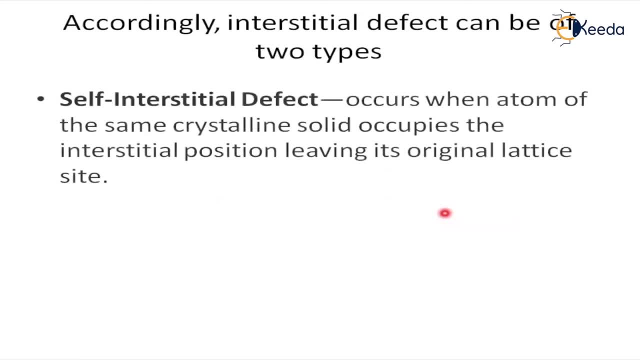 two types are adjusted. one is a self interstitial. if the same autumn occupies, then we can say that it is a self interstitial effect. if the foreign autumn occupies, then we can say that it is a interstitial, general, interstitial space. if the warm autumn occupies, then we can say that it is a 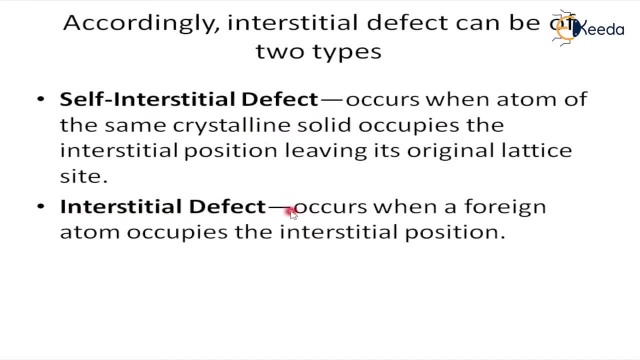 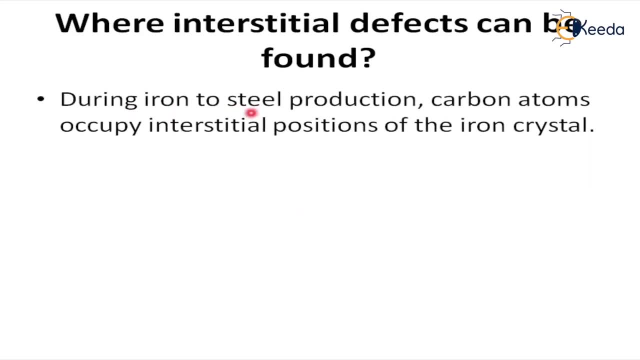 interstitial defect. now, where these defects are found, we can say that the first point is during iron to steel production. this is the main point here. carbon atom occupies interstitial positions of the iron crystal. we are finding this particular problem almost in all the materials, that is. 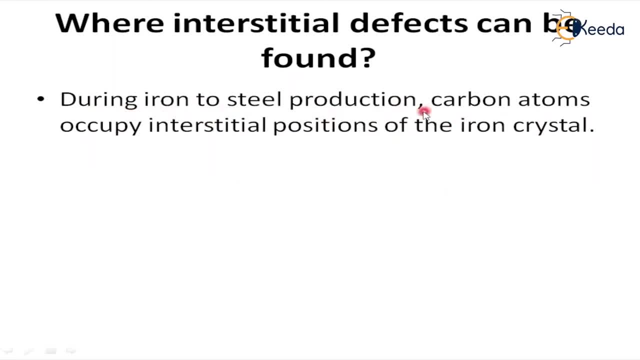 whenever the iron to steel production is existed, carbon atoms occupies the interstitial position. this is the regular problem and we are utilizing the carb, this type of property. when carbon occupies that interstitial position, the property of the material changes and that is the useful property only. similar thing happens in many allies, so many allies, the same problem we can observe and 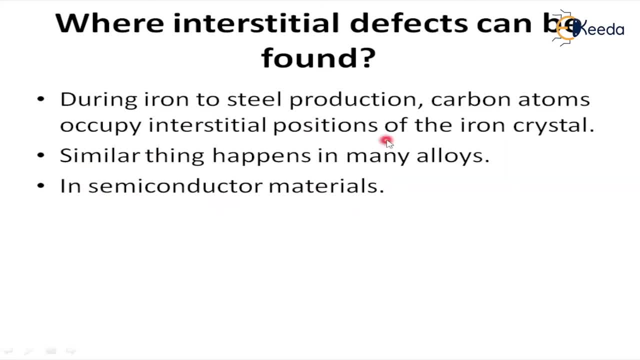 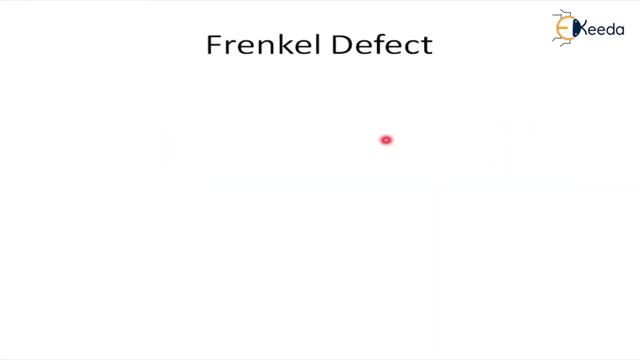 in semi neutral materials also, the interstitial defects may be observed. the next defect is franken defect. what do you mean by franken defect? franken defect is also a point effect. in fact it is a combination. it is a combination of both vacancy and interstitial type. so how we can? 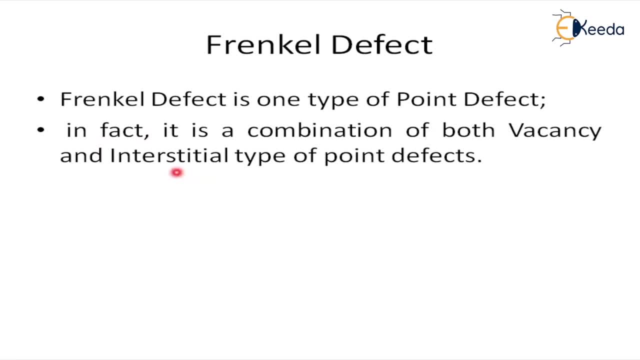 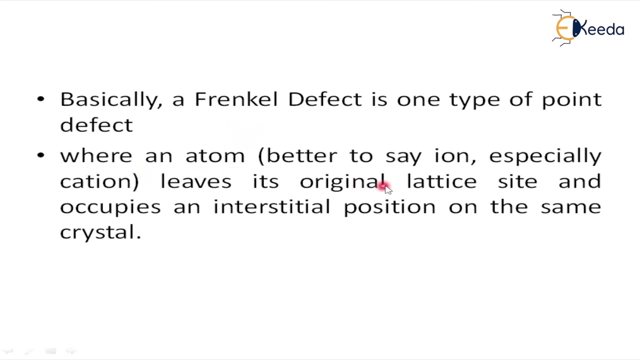 discuss this franken defect. if we're going to see the picture, see the sentence here. usually this type of defect is observed in ionics solids where the size of anion is substantially larger than size of the cat. here is a normal observation, if you observe the pain point here. basically, a franken defect is wherever so you can. 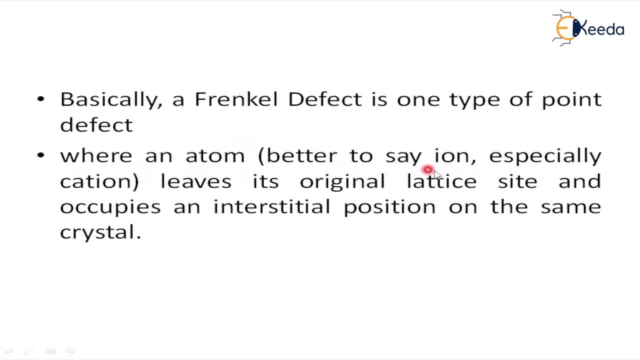 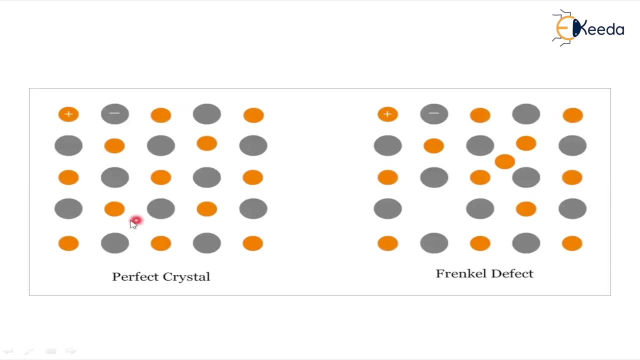 say that better to say iron instead of autumn. better to say iron because we are discussing Frankel. defect means it is a ion. in general it is an iron leaves its original lattice site and occupies an interstitial position. so that means observe. the picture here is almost like the previous one. here you are observing. 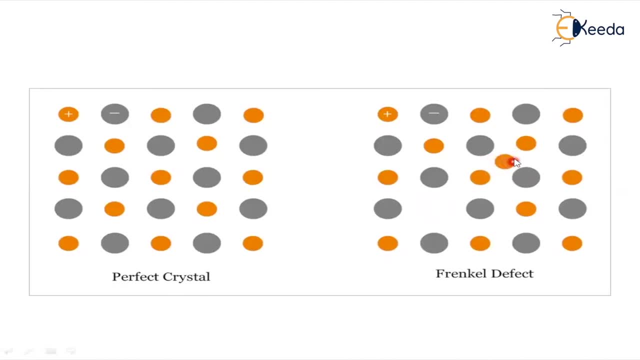 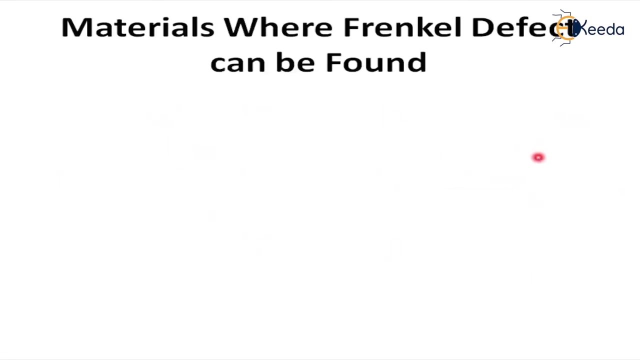 vacancy. here you are observing the occupation. this is a perfect crystal. that means this defect can be say that vacancy and occupation interstitial. so that's why this Frankel defect is represented as vacancy and substitutional, our interstitial defect. now, materials. where are the? what are the general materials we can found the? 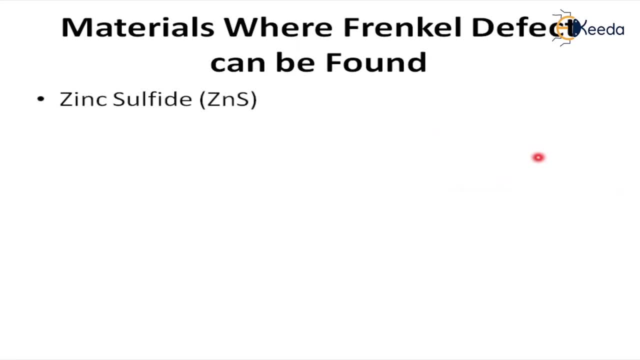 Franklin effect. please observe: one is zinc sulfide, the next one is silver chloride, the next one is silver bromide. here, all these defects are about point defects only. hope you understand the topic. this is very, very important topic without which we cannot analyze the materials. if you understand the point. 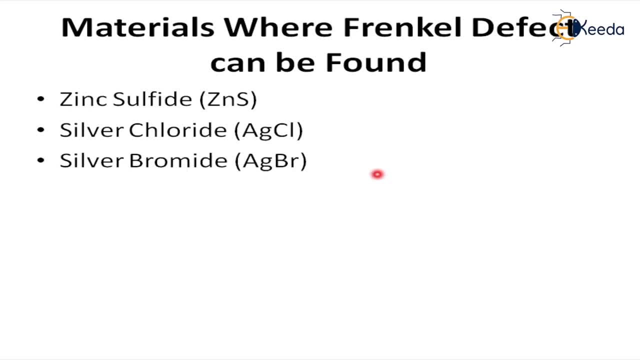 effects. then we can utilize the materials in a proper manner. thank you. thank you for at all.